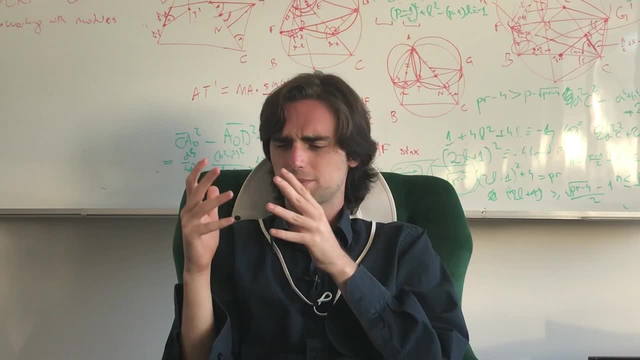 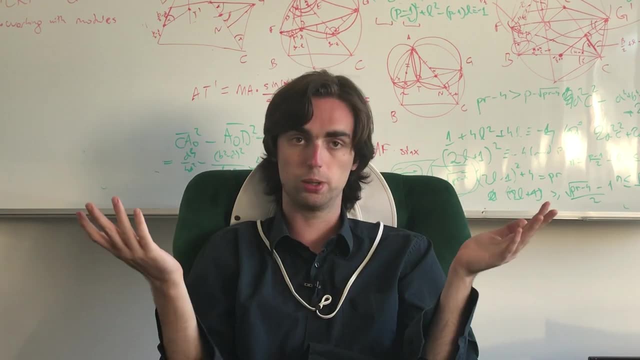 If the first two things are true. So it needs to teach you that What is divisibility? If A divides B, then there exists an integer K, such that A times K is B. That's what it is. It needs to tell you about the Euclidean algorithm, about remainders. 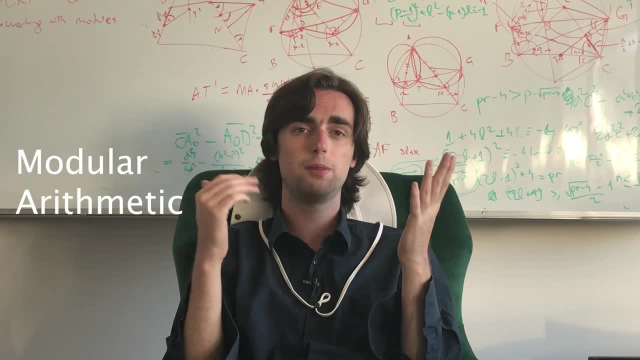 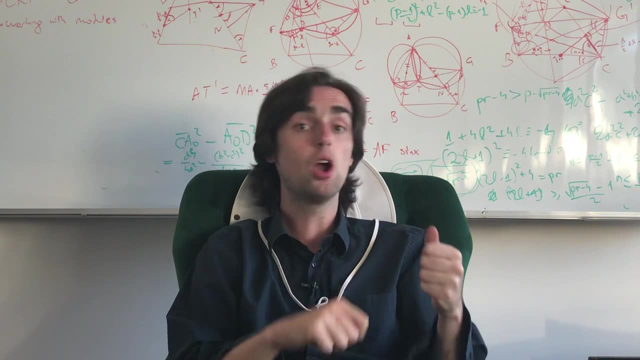 And talking about remainders, it needs to talk about modular arithmetic. It needs to mention primes somehow, somewhere. If a prime P divides A times B, then it divides A or it divides B, And with that you know. it needs to mention the fundamental theorem of arithmetic, if not prove it. 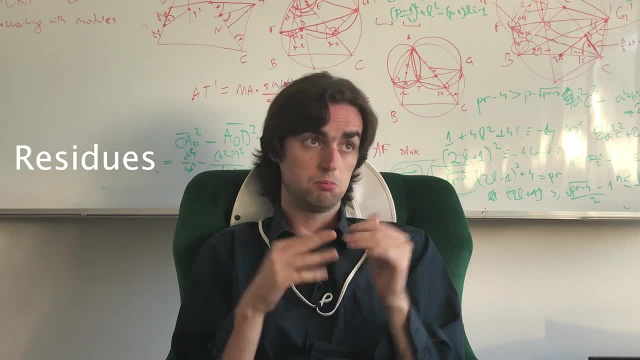 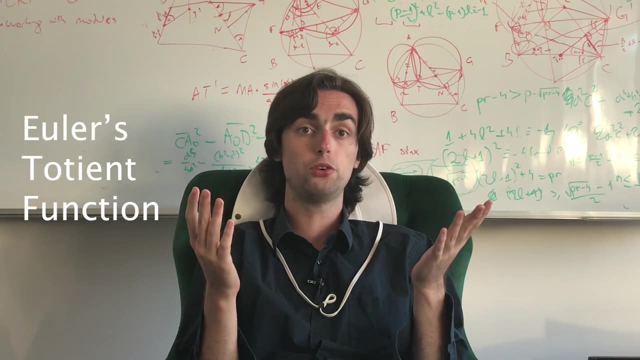 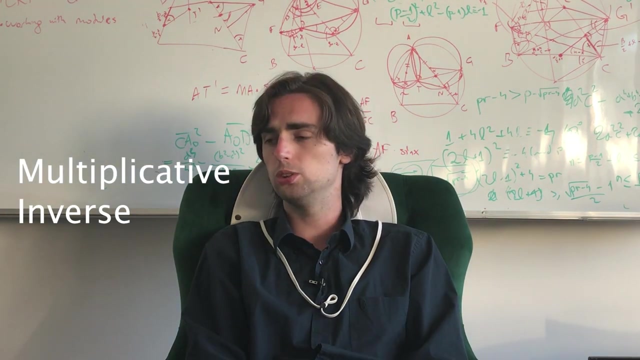 Aside from that, You also need to look at residues, quadratic specifically, but in general, when you're trying to say, prove Euler's tuition function or Fermat's Little Theorem- which it also has to mention- Inverses with residues. 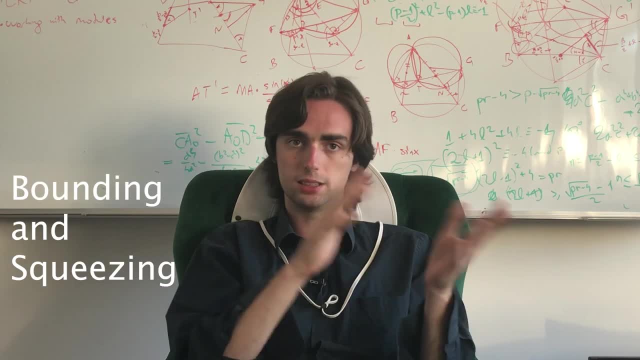 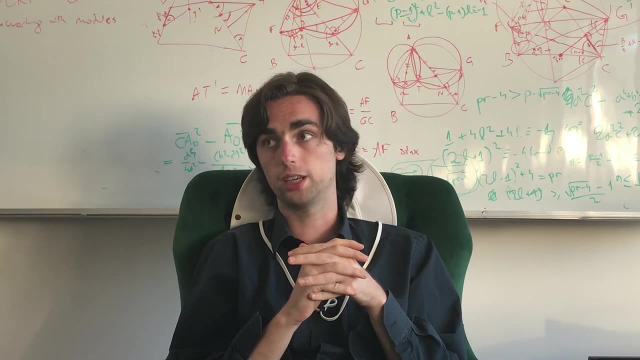 And it needs to talk maybe a little bit about bounding stuff. You know how do you prove that K squared plus K is only going to be a square for an integer K If K is equal to 0 or minus 1.. How do you prove these things? 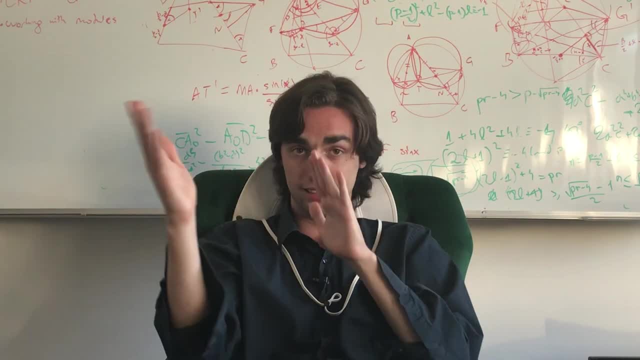 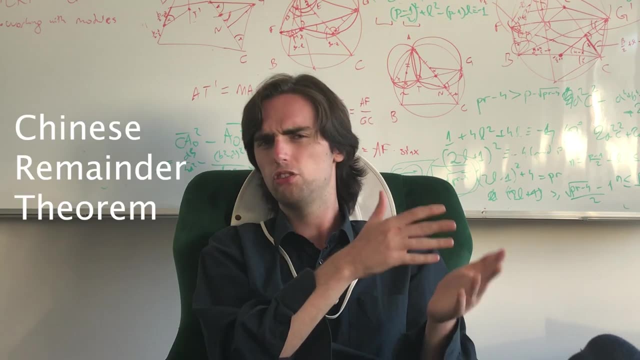 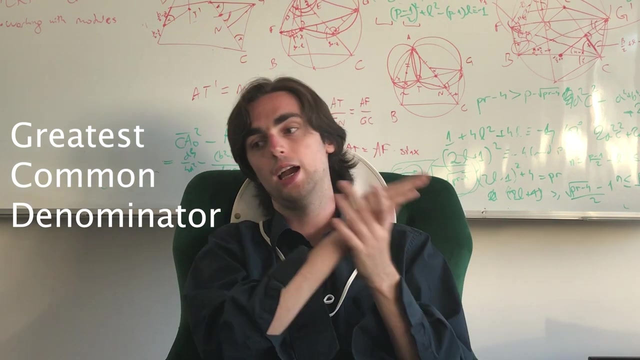 And actually is it only those two cases? It might be, but it has a bounding argument there, Or what else does it need to teach you? It needs to teach you, I think, that Chinese remainder theorem, perhaps as well: GCD, and like the greatest common denominator and the least common factor. 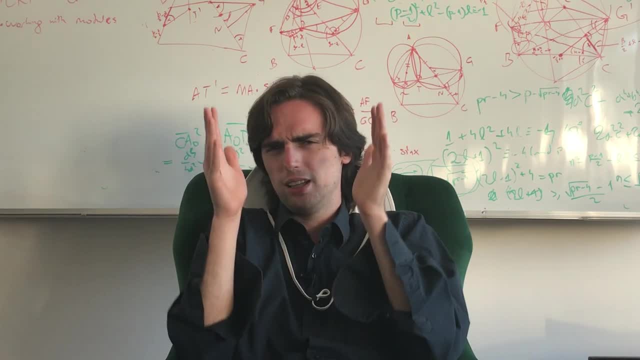 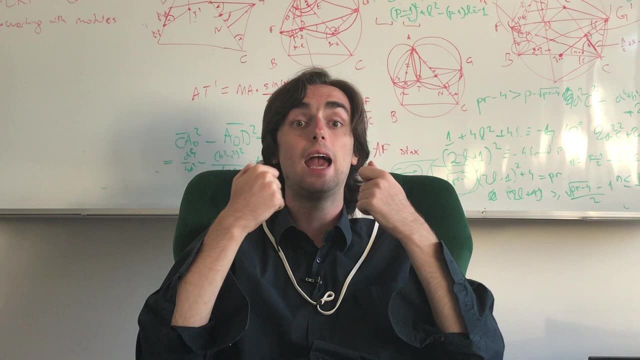 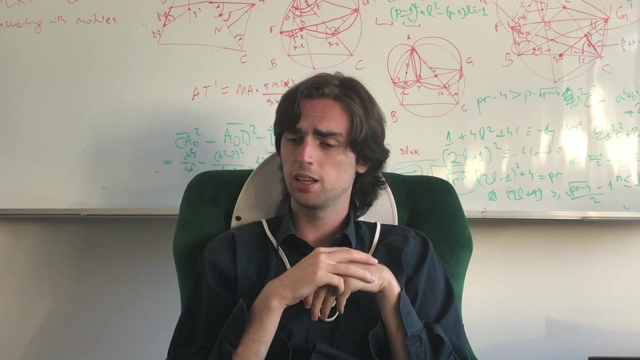 Like: these are the things that it really should teach you, Like, if you. If it has all these things together, then it's good enough. It just needs to teach you some basics and hopefully, show you some problems. The book I saw that's freely available online at the time of making this video was Justin Stevens' book on Olympiad number theory. 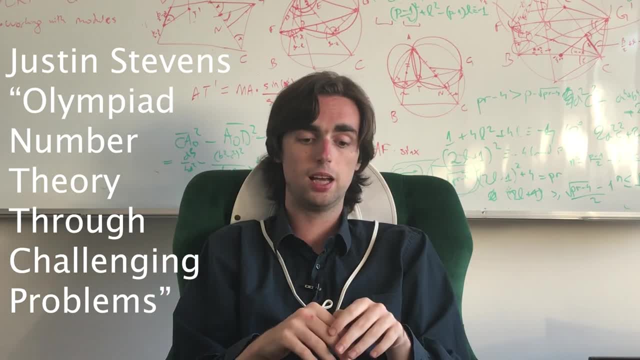 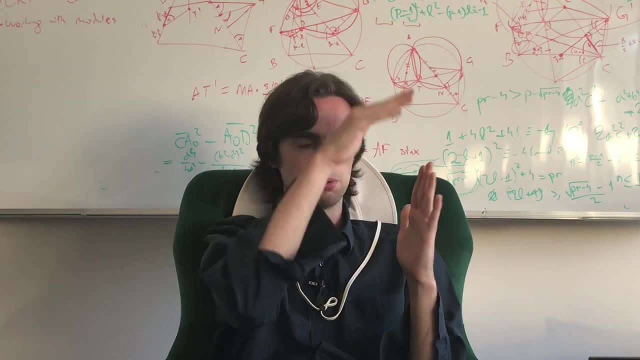 So basically, what you can do is go on your search engine and type Olympiad number theory. Take the first one, two, three textbooks. Look at the table of contents. Does it have all these things I mentioned? I'll give you a list in the description. 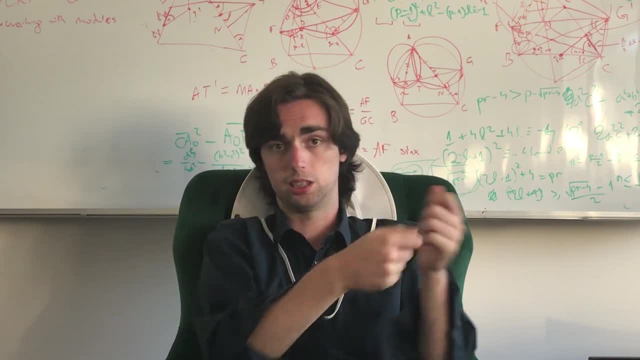 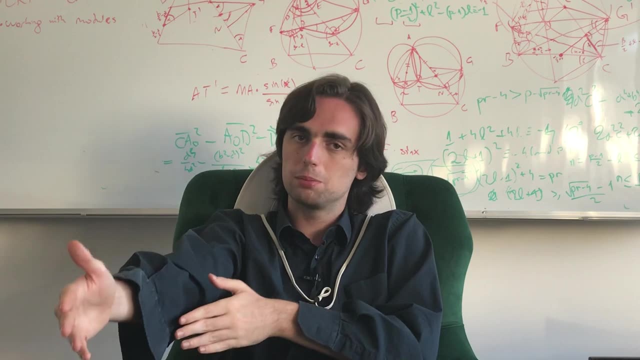 And if it does go through it, If it misses a couple of things still, you know, go through the things that it has and learn about them, And then you try to solve problems. And then you go back to the textbook- solve problems. go back to the textbook- solve problems. 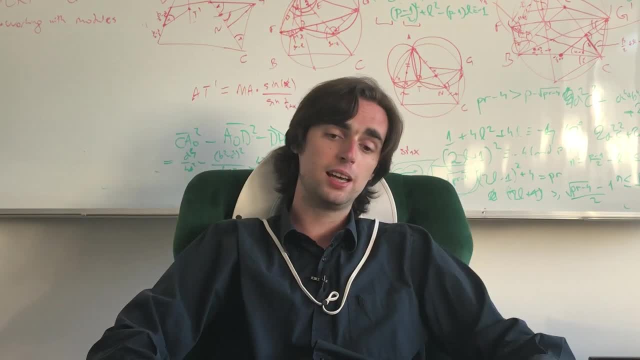 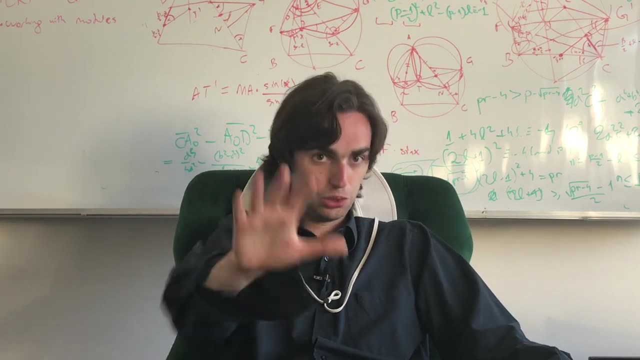 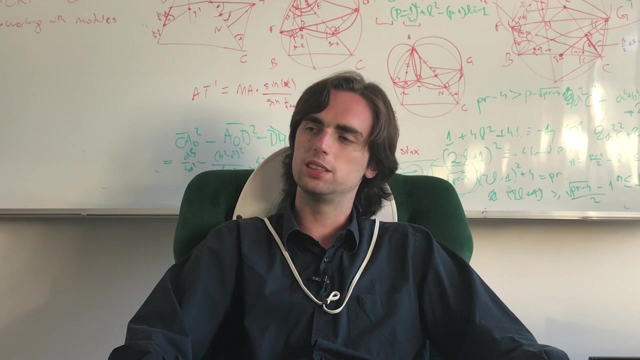 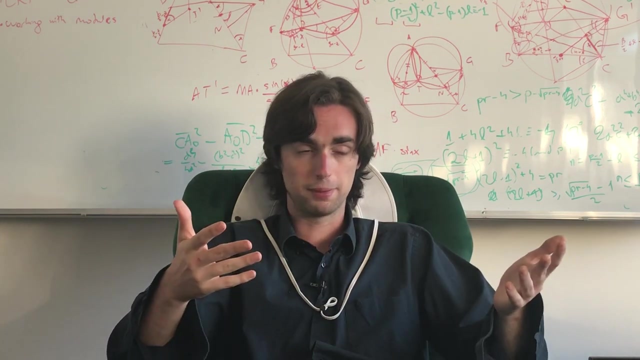 That's really the process here that you're doing, And after a while you may be looking at more advanced number theory concepts, Which I suggest you Hold off until you've gotten really good at these basic concepts. But when that time comes you can go on, say, Evan Shen's website and look at his maybe handouts or his suggestions for number theory. 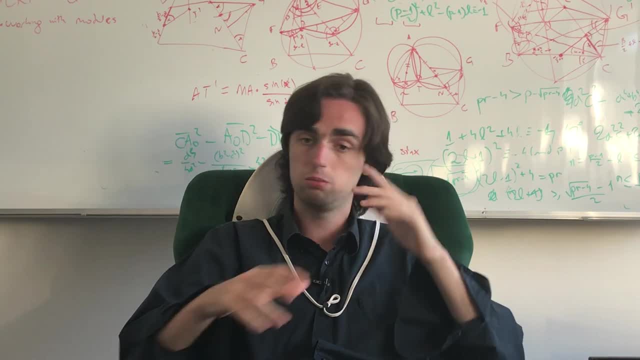 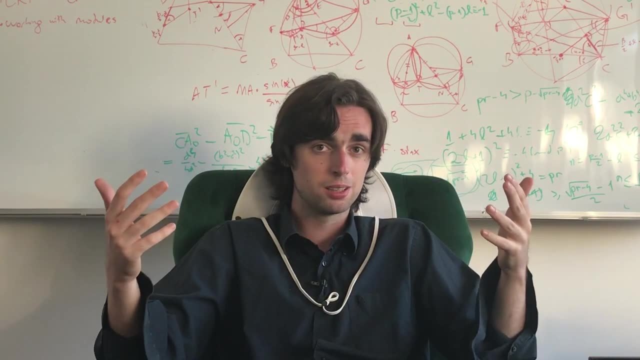 He has phenomenal Olympiad suggestions in general And with that that's really all you need to solve number theory problems and to learn the theory behind number theory- One textbook or a couple of them. They really just need to mention all these things. 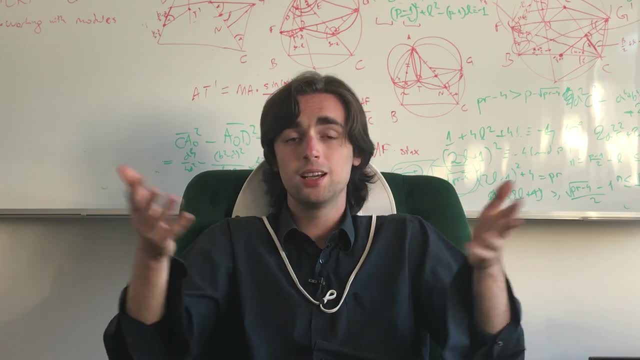 All these concepts show you a couple of problems, so you're familiar with them And with that you're set And, as always, thanks for problem solving. 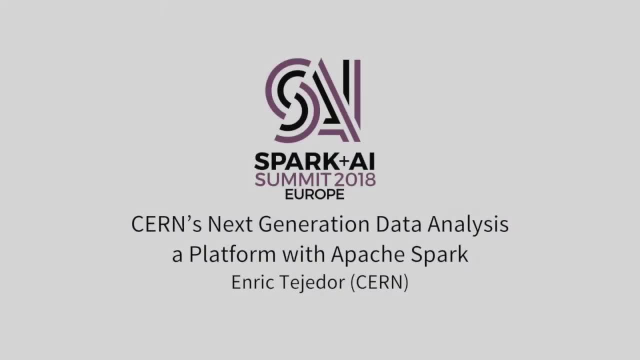 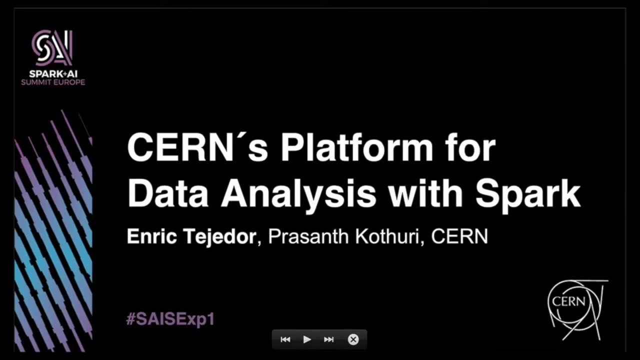 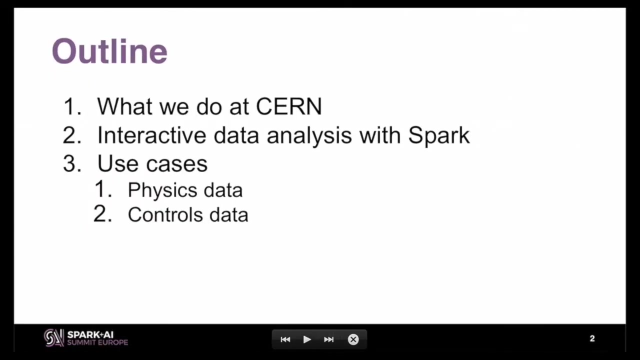 Good morning everyone. I'm Enric Tejedor. I work at CERN, in particular, in a group that is called SFT that takes care of software development and support for the experiments at CERN, And I wanted to tell you about an interactive data analysis platform that we 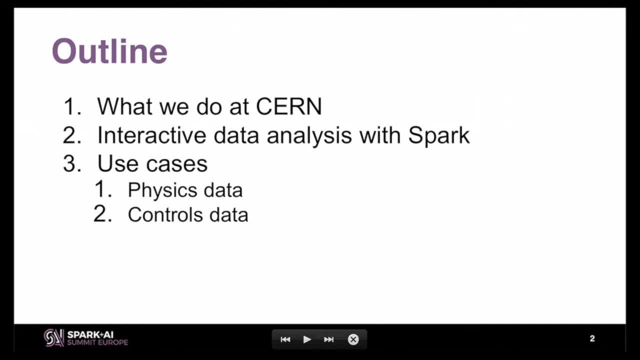 have at CERN that is called SWAN, which physicists can use to do data analysis by uploading also computations to Spark clusters, And I will present a couple of use cases of groups that are already using this platform to do analysis with Spark at CERN. 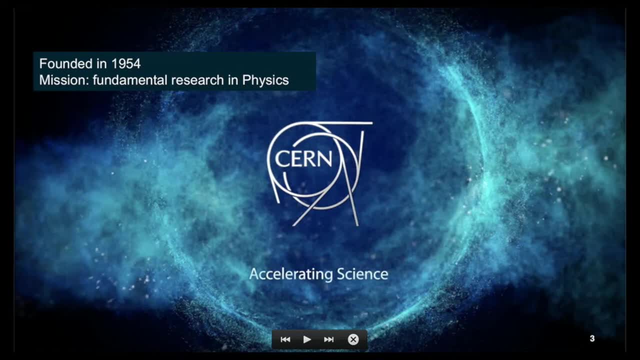 But first I will start with a brief introduction to CERN. CERN is the European Organization for Nuclear Research. It was founded more than 60 years ago already With the mission of doing fundamental research in physics. So we study the basic components.